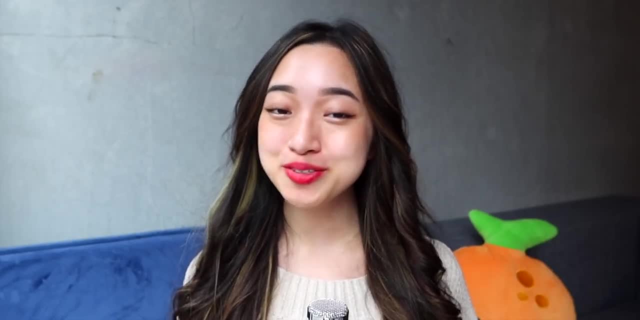 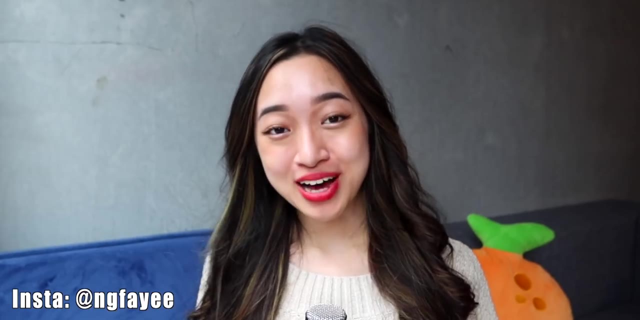 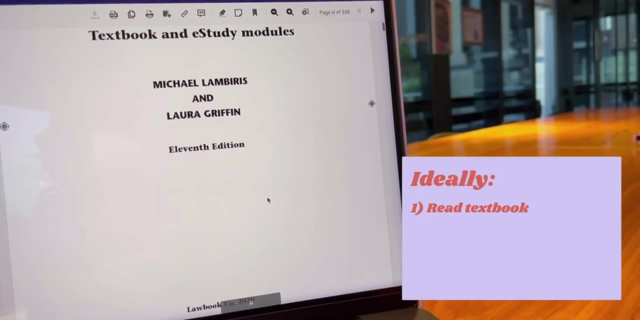 Then be sure to watch till the end of the video to know what that study tip is. First skip the questions. copy the answers Now. I'm not asking you to cheat during your exams. okay, Basically, during revision, you ideally want to read your textbook first. 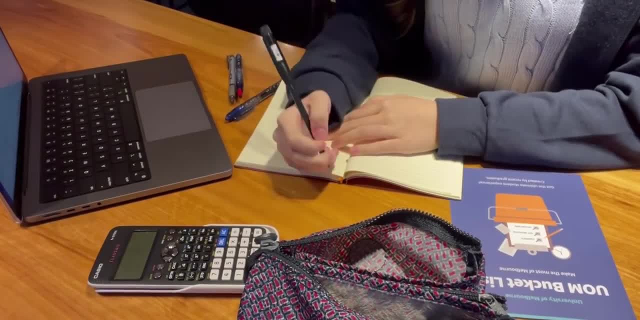 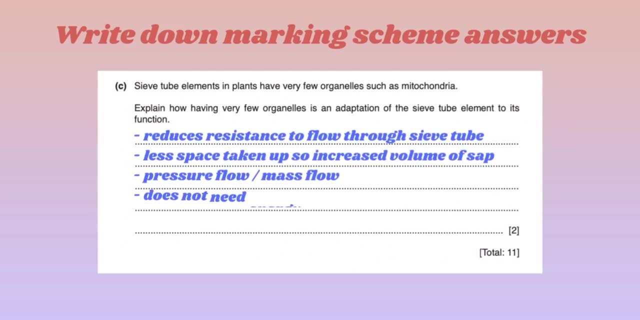 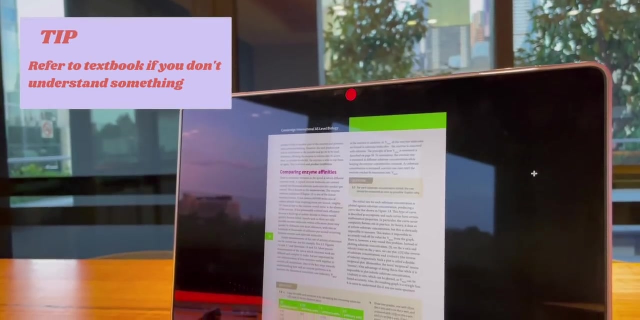 then do questions. But if you seriously have no time, take your past year papers or sample questions and just write down all the bullet points or answers from the marking scheme Study. these model answers Only refer to your textbook. if you don't understand anything, 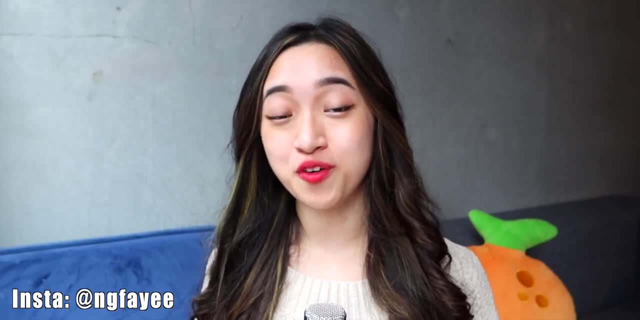 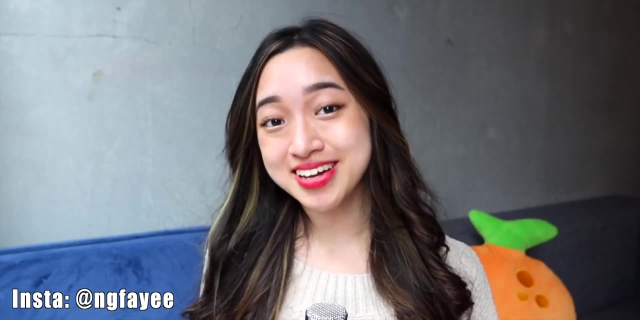 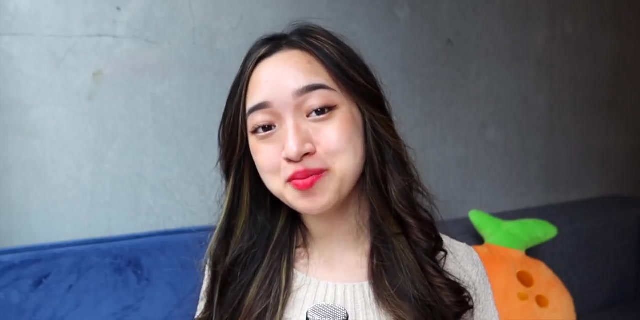 to save your time. I usually do this a day or two before exams if I just want to reinforce some extra knowledge without having to do questions. But this study tip is also really effective. if you don't know anything and you want to cram, You'll automatically be studying exactly what the teacher or marking scheme wants. 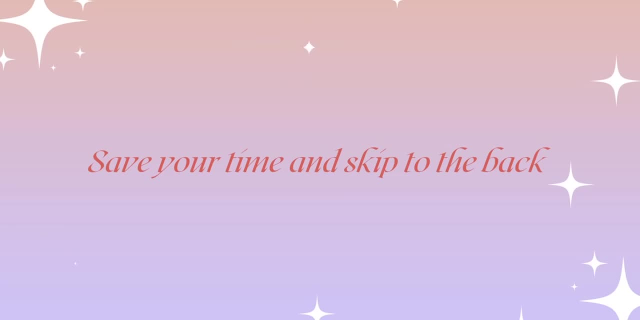 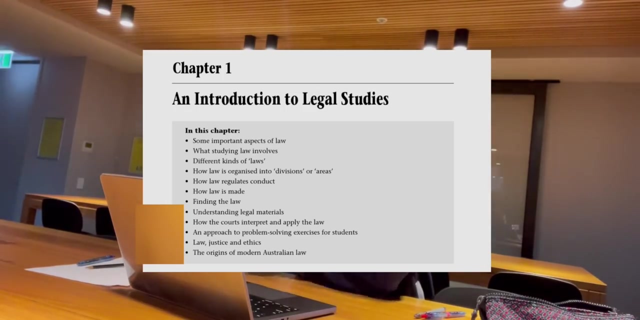 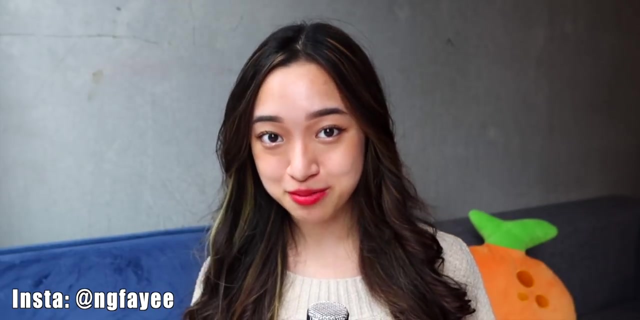 Next, save your time and skip to the back. In the beginning of each chapter of every textbook, there will be a section outlining all the key points in the chapter. This is not what we want to focus on right now, because we are rushing- I've mentioned a few times before- to focus on the learning objectives. 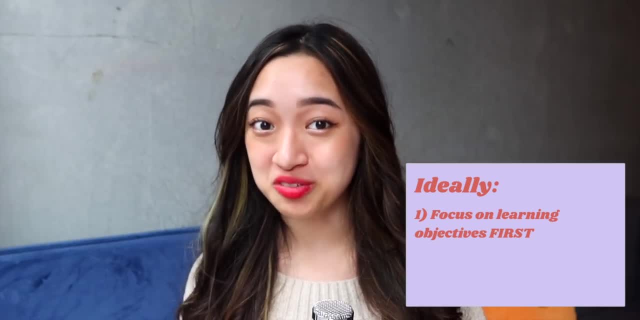 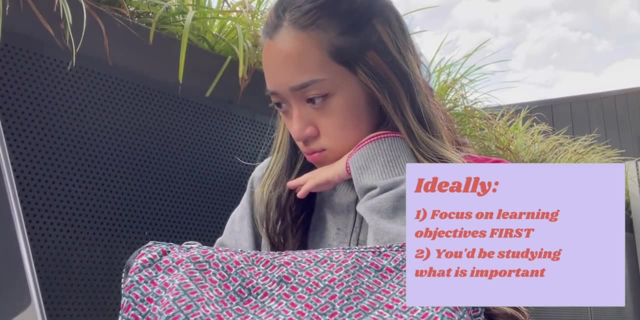 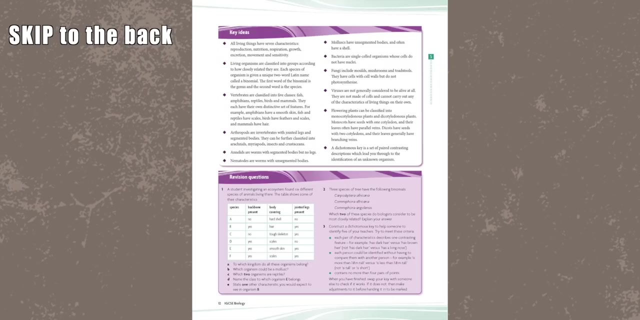 when studying a subject, And this study tip will already save you a lot of time, because you'd just be studying what is important in the chapter first before moving to other parts. In this case, since we're cramming for exams, just skip to the back of the chapter. Usually, there will either be a list of questions, they 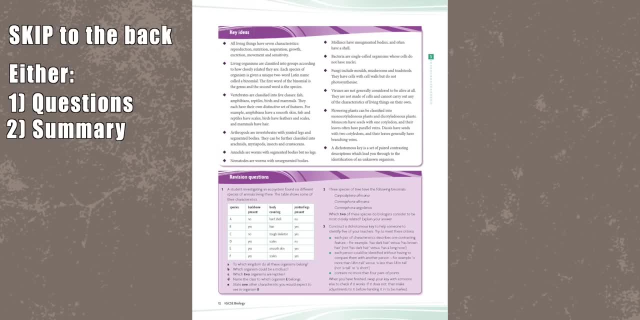 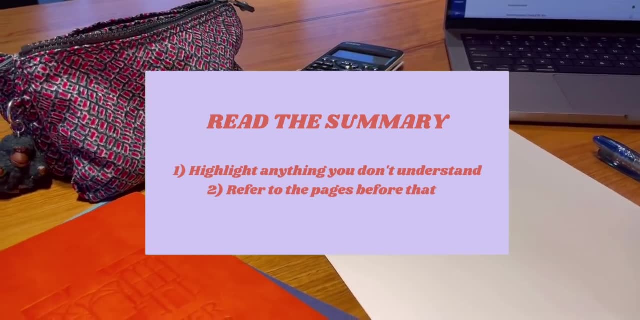 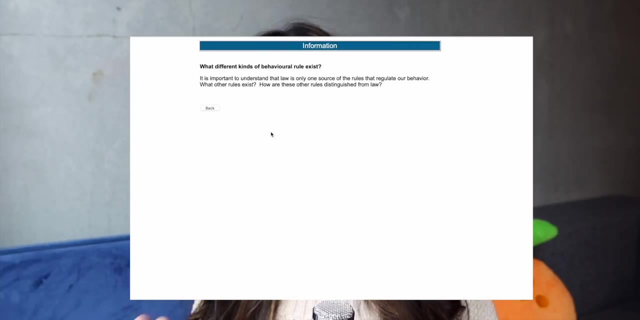 want you to answer, or a summary of the entire chapter. Read the summary, highlight any keywords you don't understand and work backwards from there. If there are questions, answer the questions. A lot of the time the exam will just pick these questions, then twist and turn. 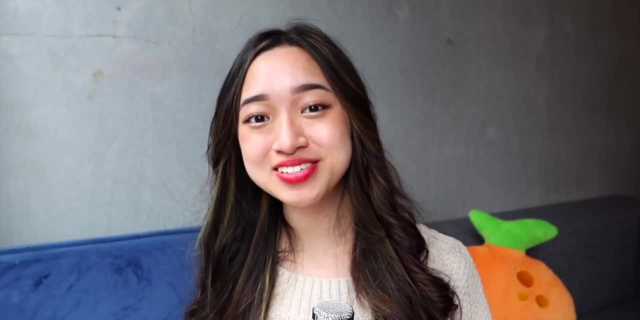 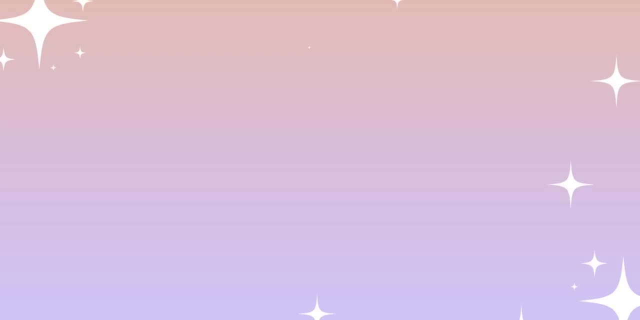 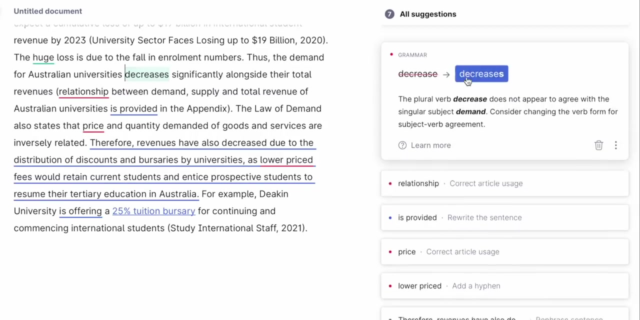 The way they ask them, but the concept and the answers are similar, So take advantage of the last page of every chapter. Next, another time saving tip: I'll tend to write a lot of essays when exam season is coming And if I want to get them. 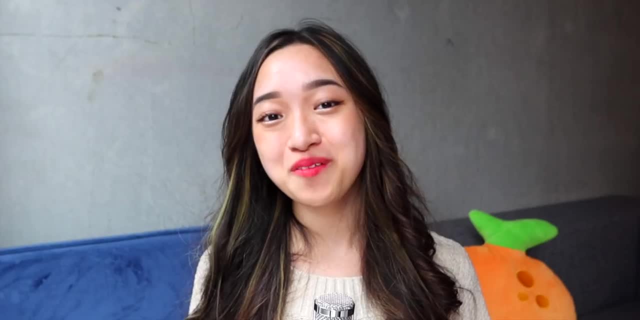 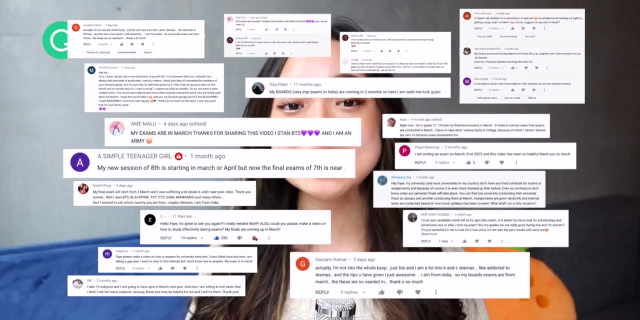 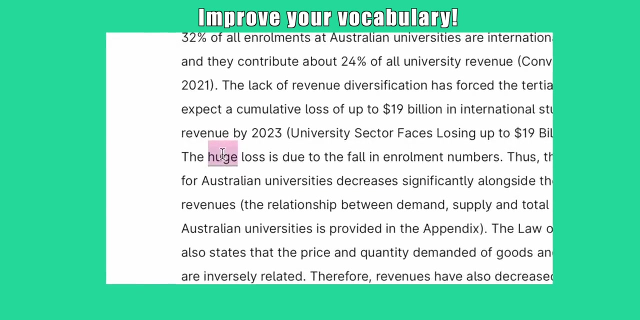 checked super fast. I just use Grammarly. I've been using Grammarly since secondary school because it's free And since a lot of you are having exams in March, this tool will also help expand your vocabulary and improve your essays, as it has premium vocabulary suggestions that will 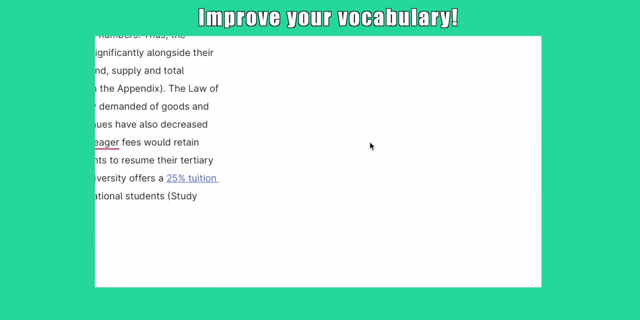 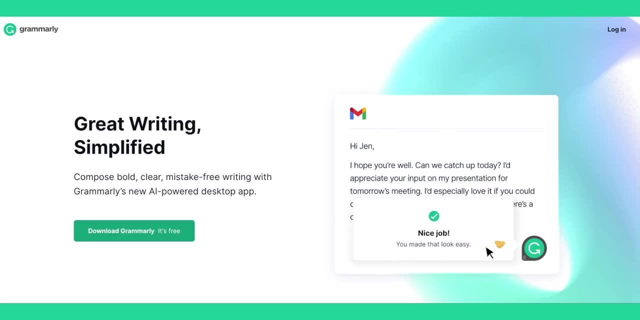 replace your boring words with better ones. Basically, Grammarly is a digital writing assistant that improves your writing, helps you be more productive and saves you time. Just download Grammarly into your desktop, then you can use it anywhere, such as Google Docs. 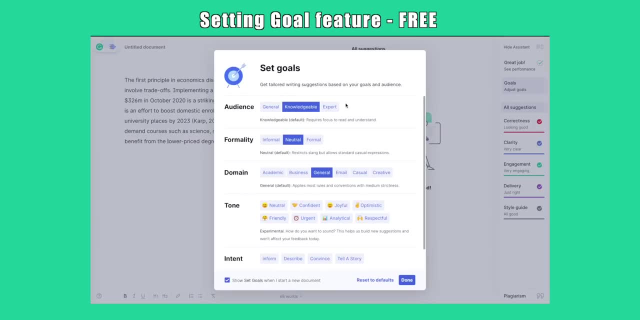 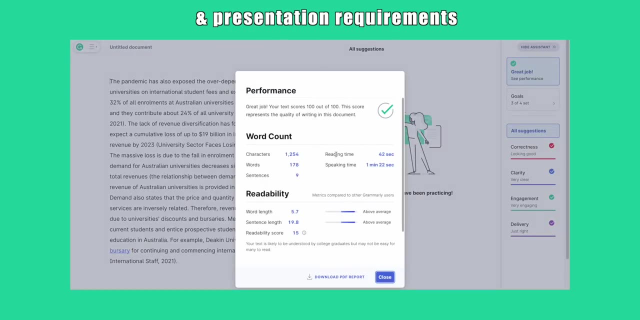 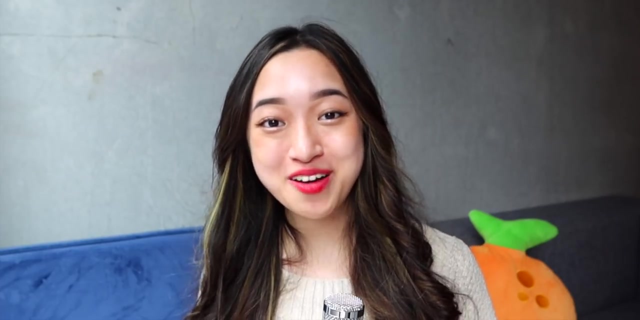 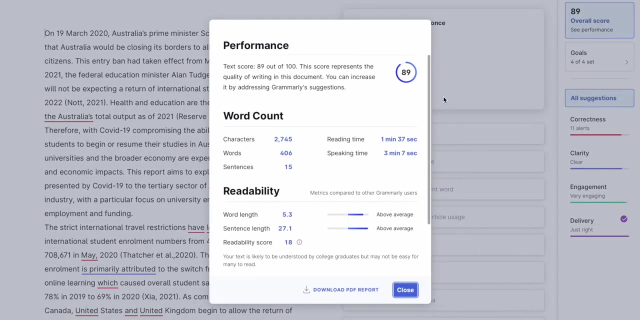 The setting goal feature ensures that everything you write has the right tone and formality. It makes sure that you meet your assignments and presentation requirements, as it helps calculate reading time, speaking time and vocabulary. I seriously use Grammarly for everything from checking my emails to writing my 1500 word essay for economics to make sure that my essay stood out. 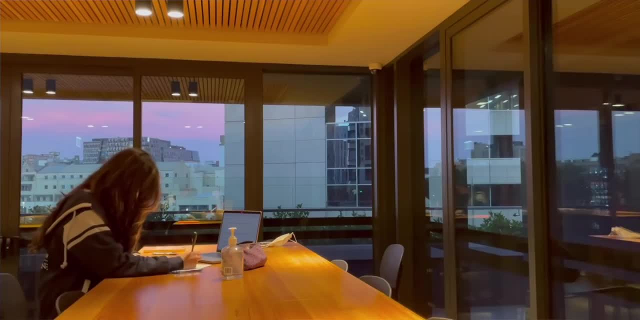 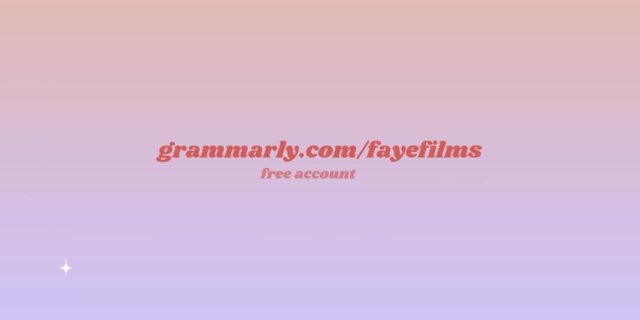 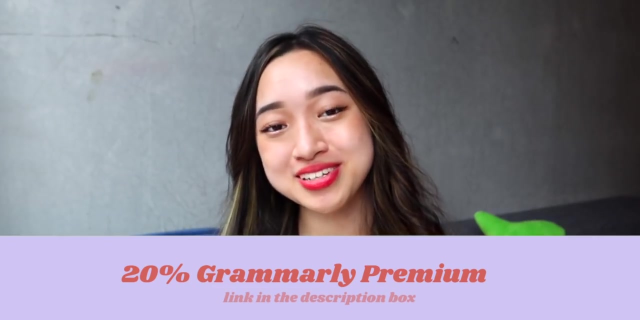 Since it's exam season and it's a new semester, make sure that you're prepared to tackle all those essays by going to grammarlycom slash faefilms to sign up for a free account And if you want extra features such as premium vocabulary suggestions, upgrade to Grammarly Premium for 20%. 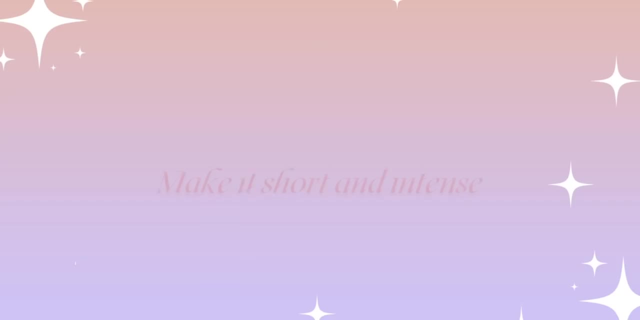 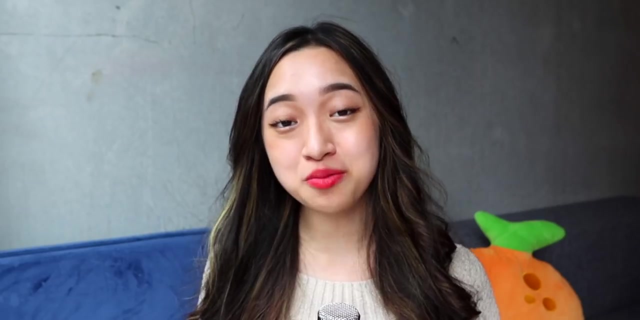 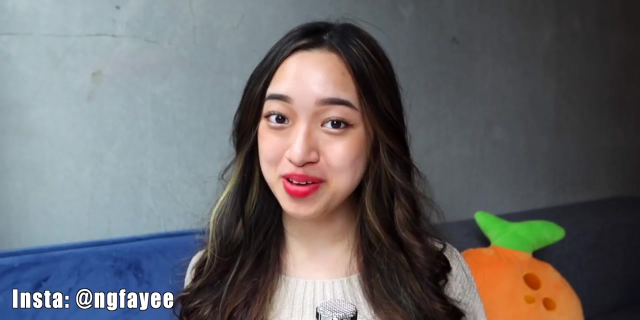 off using the link in my description box. Next, make it short and intense. I went to a lecture conducted by the University of Melbourne and they talked about a time management technique called frills: Frequent, regular, intensive, limited sessions- Basically, if you want to do a study. 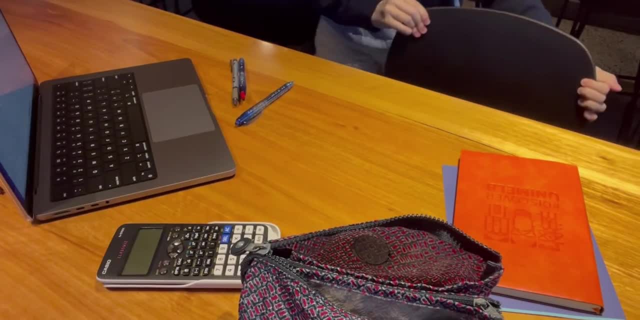 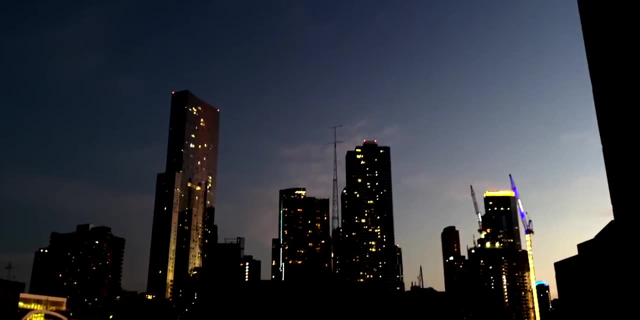 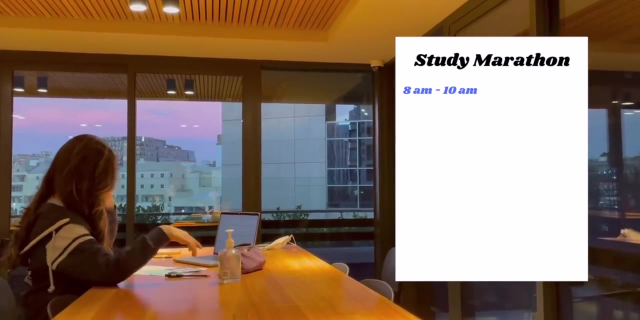 marathon where you study the whole day. make sure that your study sessions are short but intense. That way you'll have the stamina to sustain until the night. So let's just say you want to study for eight hours in a day. You study for two hours first, from 8 am to 10 am, rest for 30 minutes. 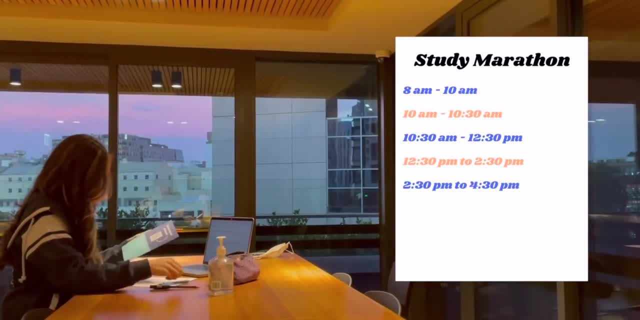 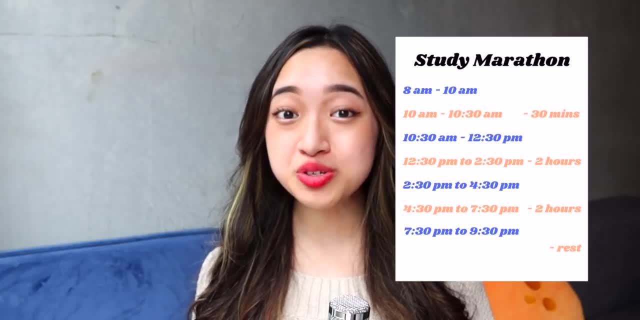 study again for two hours, rest for two hours, study for two hours again, then a three hour break. Get this: You studied for eight hours, but you also had more than five hours of rest time. How amazing is that, If you want to study for 10 hours, your 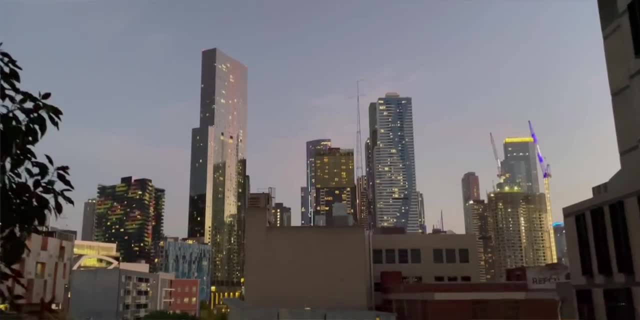 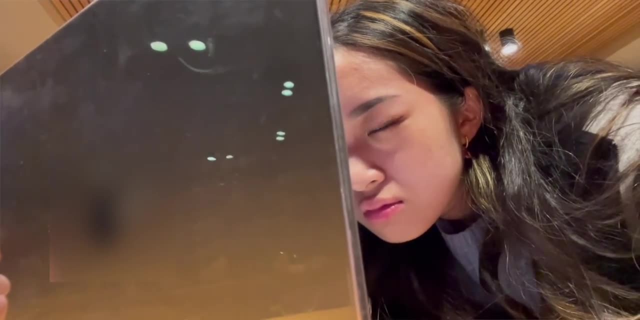 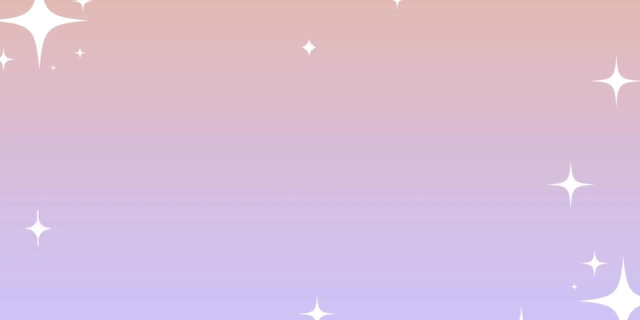 schedule will look like this: Don't try to wake up at 6 am, then study until midnight with no breaks. Your brain will turn into mush and your eyes will fry off. If you want to know how to focus when studying and stop daydreaming, then check out my video here. Next videos and cheat sheets: 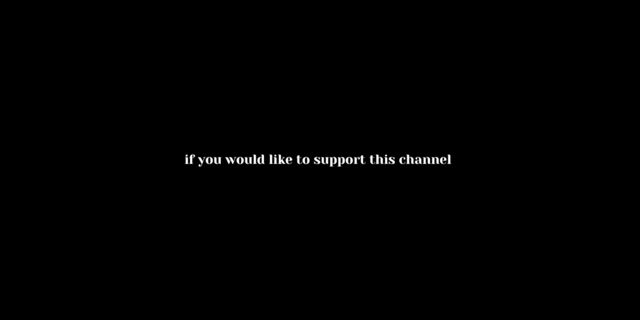 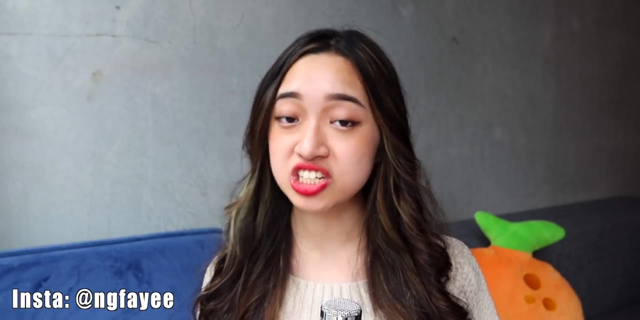 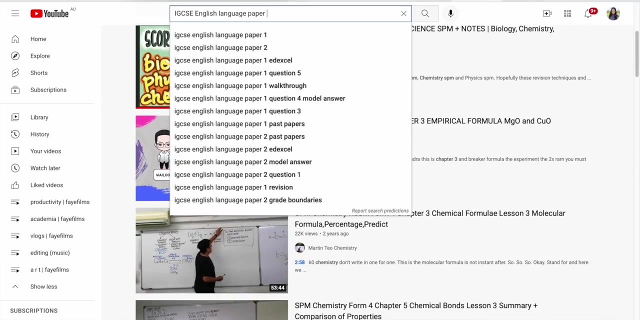 An advertisement might play in the next few seconds, so if you want to support this channel, please do not skip the ads. Thank you. If you're sitting for a big national or international exam, chances are there are a lot of videos on YouTube that explain summaries about a topic or a subject. 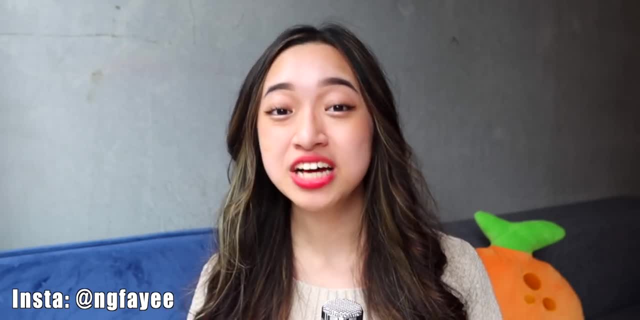 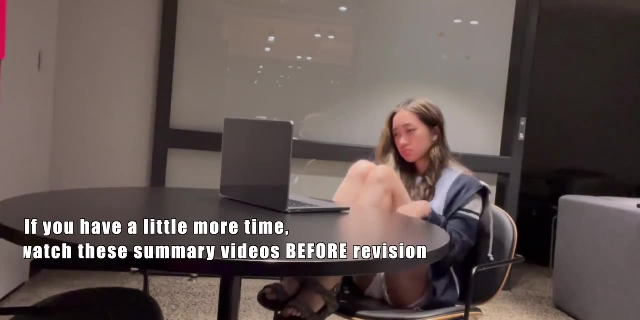 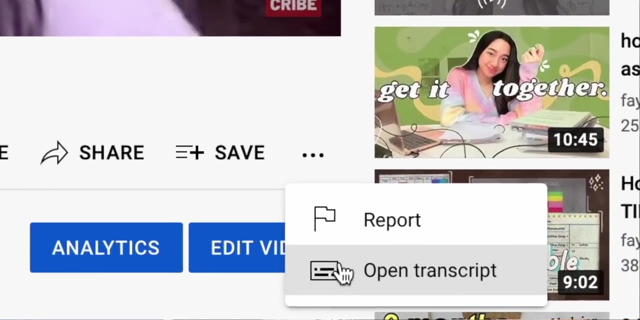 If you're trying to cram an entire subject in one day, just watch these videos. If you have a little more time, then watch these videos before you start revising, so that you do not go into revision. I hope you guys enjoyed this video. If you enjoyed it, please give it a thumbs up and subscribe if you want to see more. 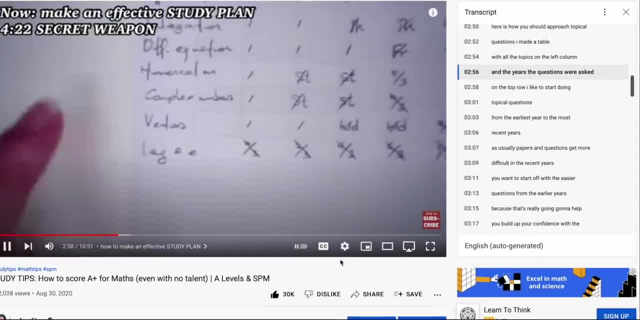 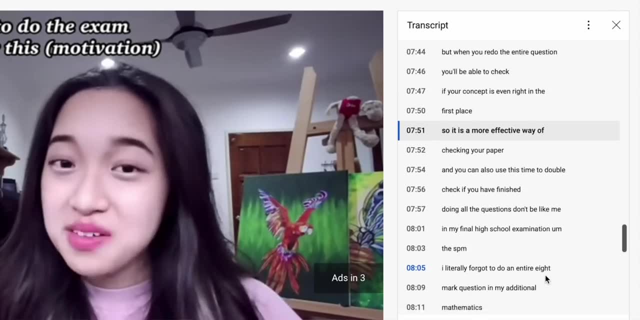 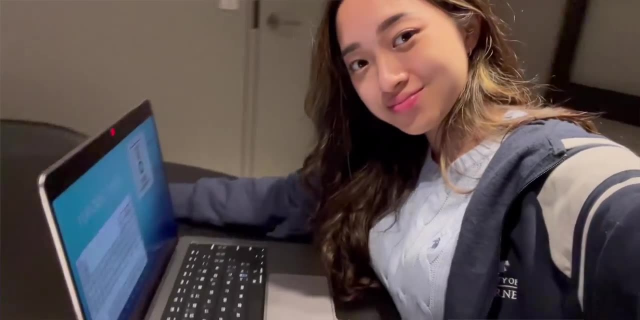 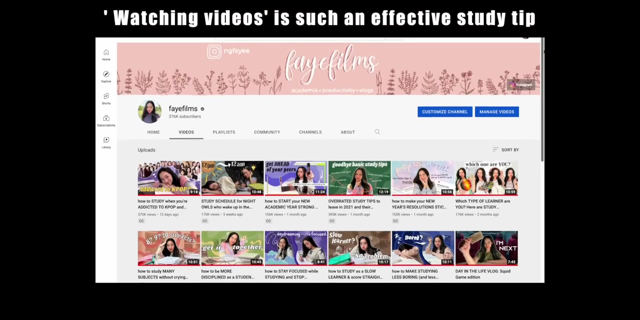 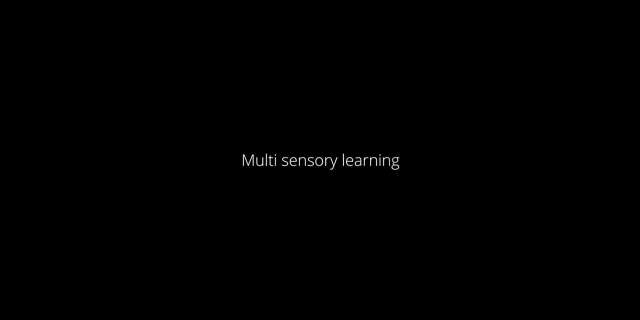 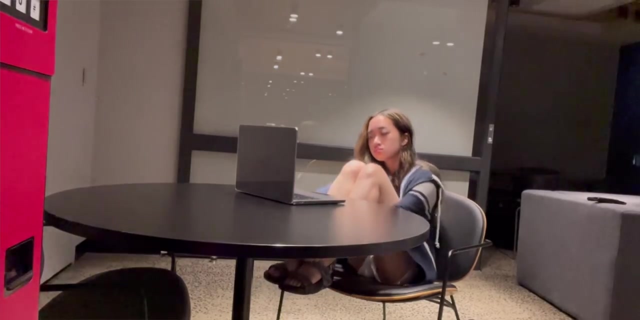 I will see you in the next video. Watching videos is such an effective study tip. You'll learn really fast because you're implementing something called multi-sensory learning, Basically by using more than one sense when learning something, in this case, watching. 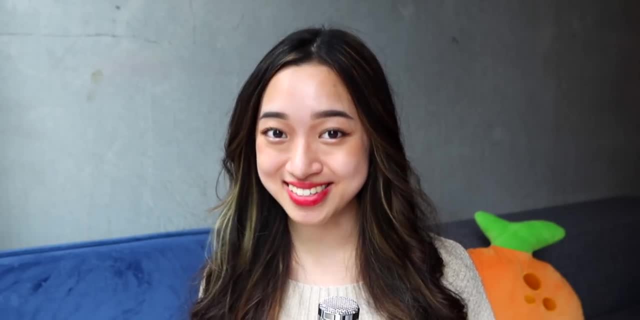 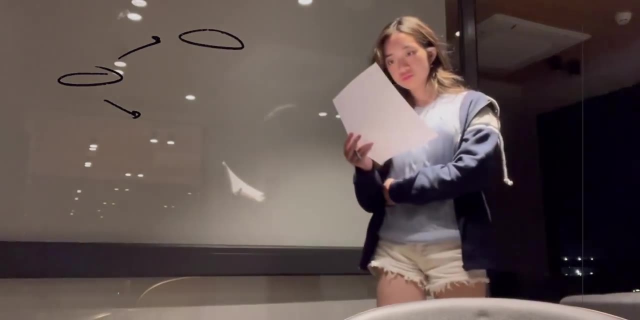 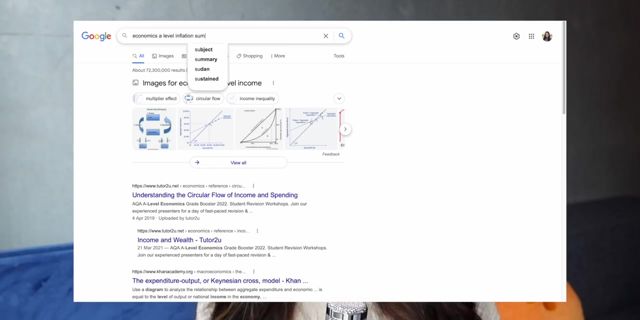 listening and writing information is more likely to stick. After you're done, go through the keywords again, without referring to the video, and make a simple mind map connecting all the concepts you understand. You can also do this: Search online for summaries of the chapter or cheat sheets. 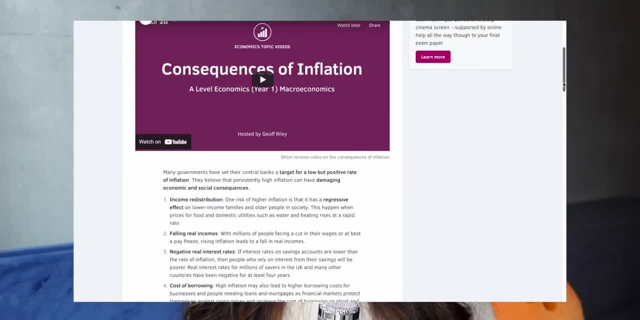 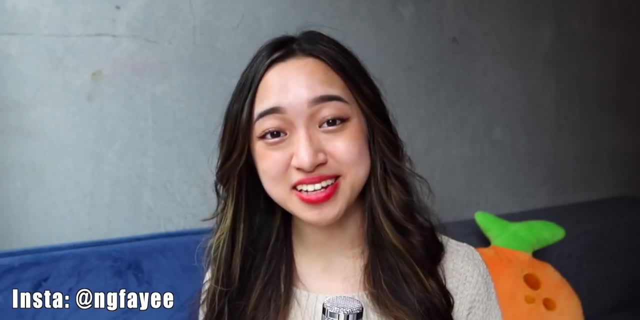 Don't do any notes. you don't have the time- just read those cheat sheets or summaries. Next, this study tip will save your exam. This is a study tip that I accidentally figured out in secondary school because I was cramming for my exams. 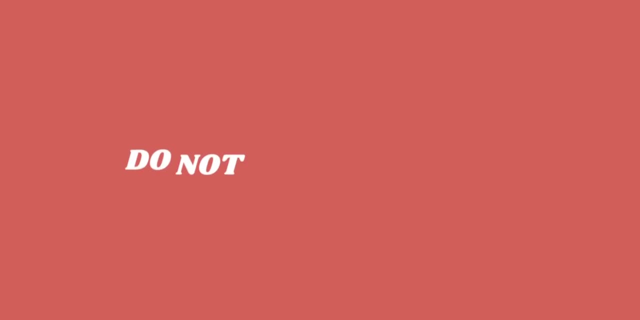 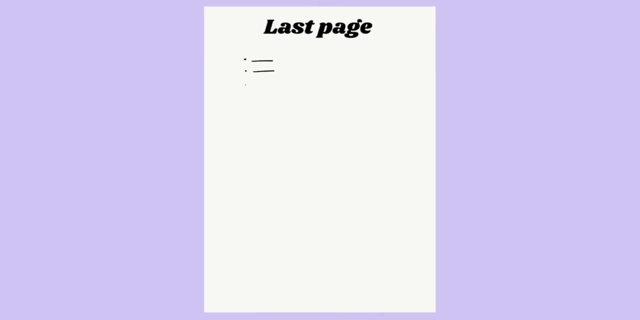 When the teacher tells you that the exam has started, do not open the paper. Flip to the right, Flip to the back. Use the first 5 minutes to dump everything that you know on the last page: All the keywords, processes, formulas, everything.